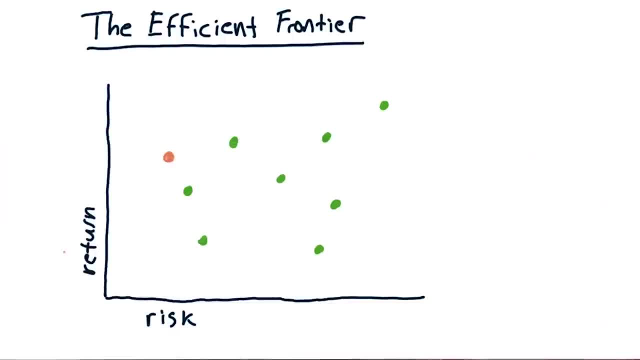 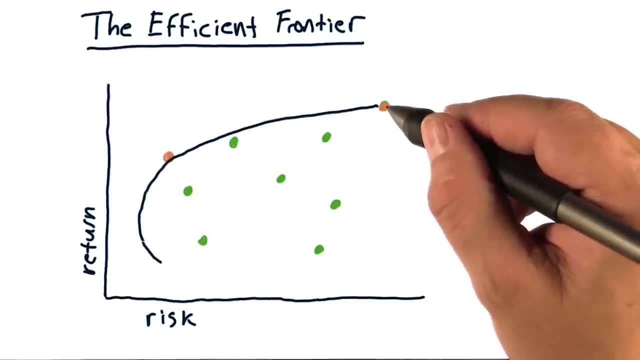 so we couldn't really do it. for all of them. you get a line, So our maximum return portfolio is up here and it would consist entirely of that one asset. But as we bring the return down, we find a number of other portfolios, all the way down to here. 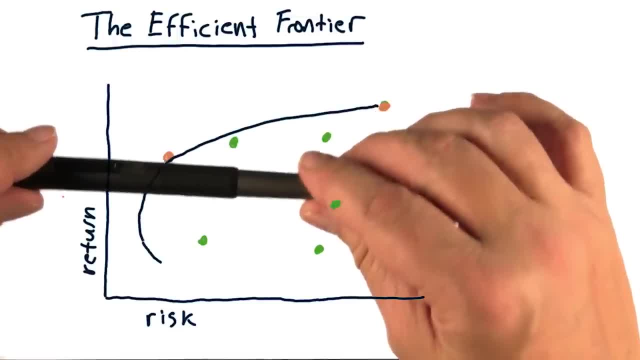 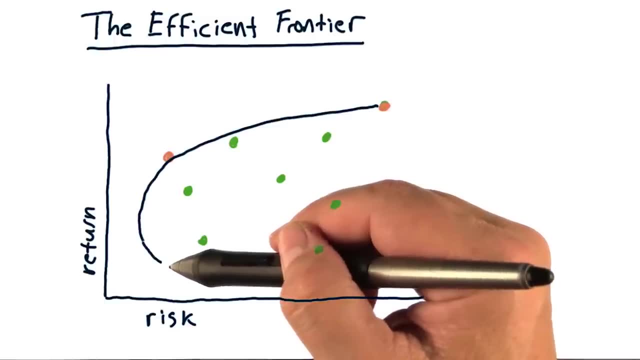 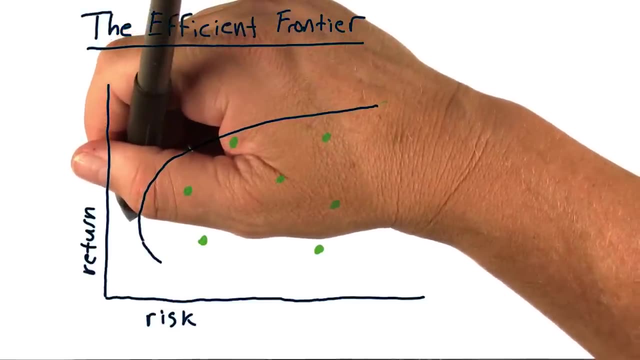 Couple different things to observe that are interesting. One is is as you reduce the return, sometimes this curve comes back in this direction, indicating that actually the risk is increasing as we reduce the return. So for the most part, people don't want those sorts of portfolios. 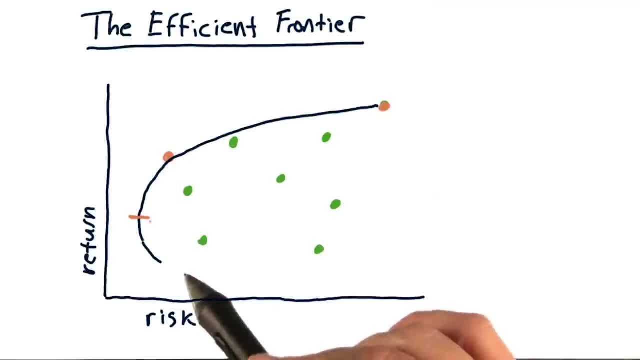 In other words, who wants a lower returning portfolio with more risk. So we typically look only at portfolios above this line. As you might have guessed, the name of this line is the efficient frontier. So what does that mean? the efficient frontier? 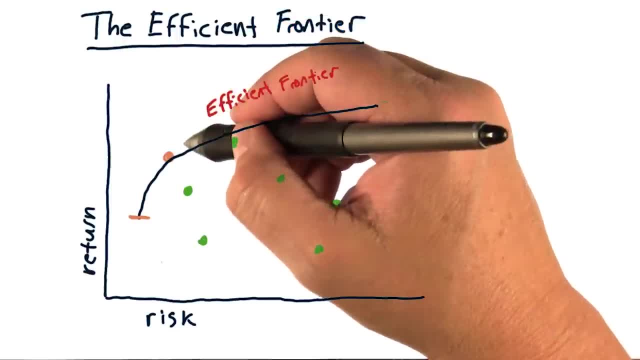 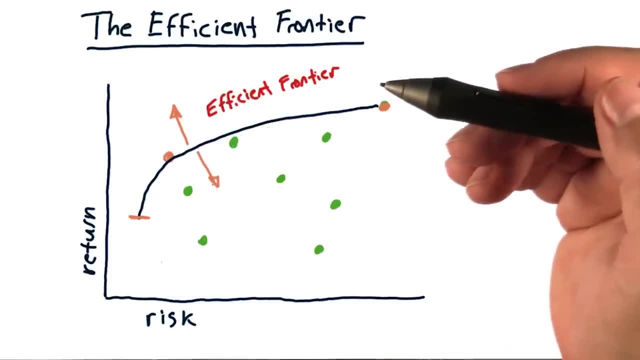 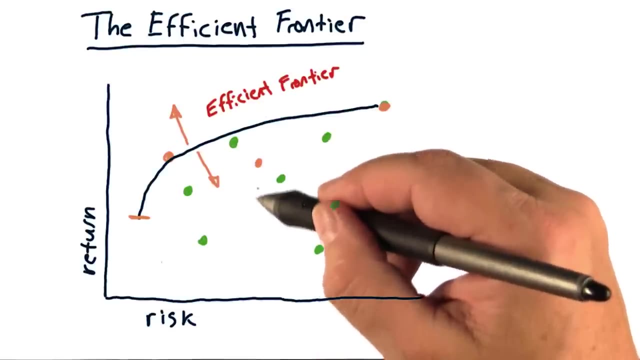 Well, it means that there are essentially no portfolios out here and that any portfolio that's on this side of the frontier it's suboptimal in some way. So, for instance, if you had a portfolio here, you are assuming this much risk for. 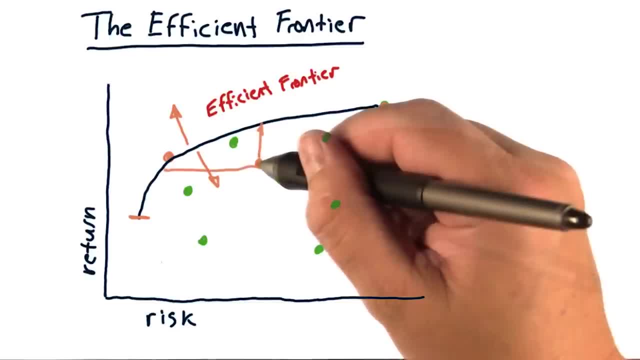 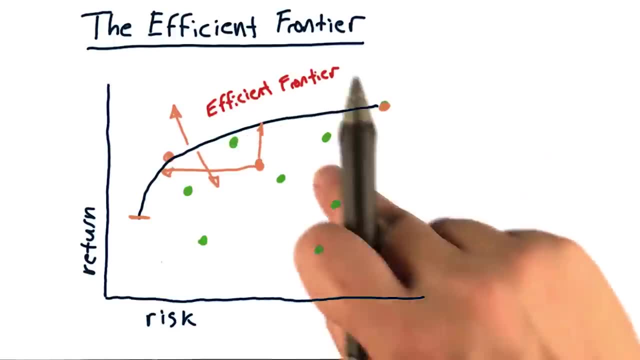 a lower return Then you could have if you were up here on the frontier, Or if you were targeting this much return, you could be over here. with regard to risk, So any portfolio inside here is not efficient because it's either higher risk or lower return than it could be if we were on the efficient frontier. 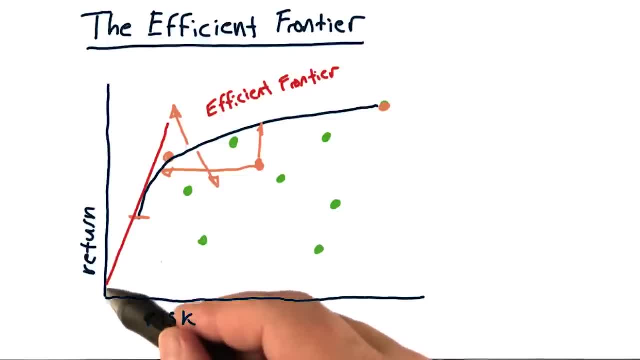 One last thing to mention about the efficient frontier is, if you draw a tangent line from the origin to the frontier, where it hits is the max and the maximum It's a sharp ratio portfolio for all of these assets. In practice, the efficient frontier isn't used for. 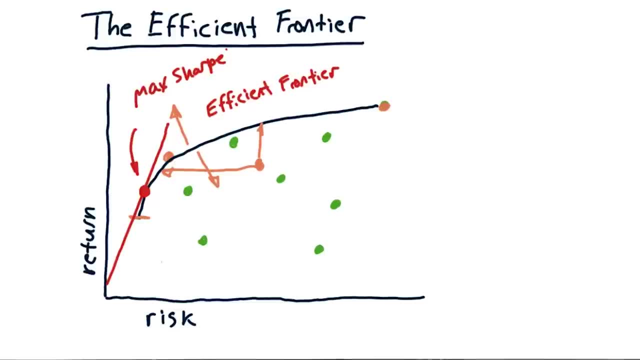 that much other than as a theoretical device, But people do often like to plot the efficient frontier so they can see where their portfolio is in relation to the assets that they're using and where they could be in terms of efficiency. Okay, that is all. I will see you online soon. Thank you very much.